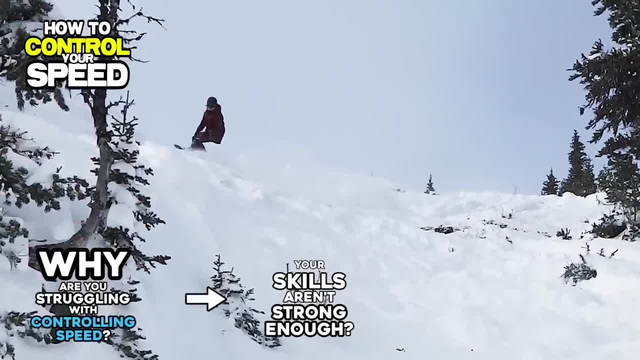 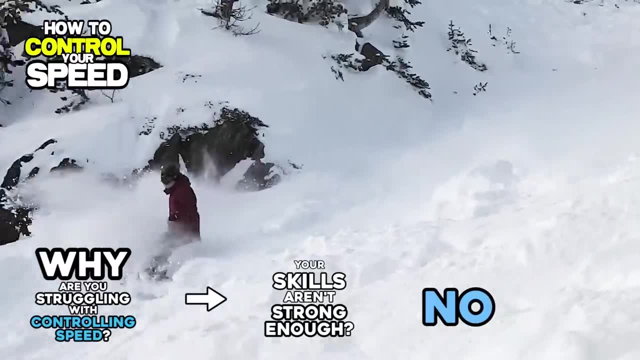 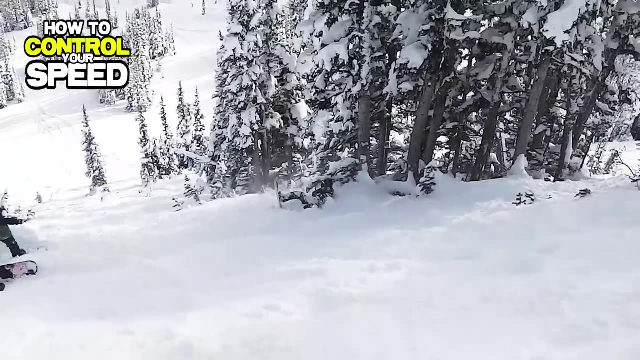 on steeper slopes. Is it because your skills aren't strong enough to control your board? No, Because my athletes who are hitting big jumps and rails on a daily basis. they still have trouble controlling speed while turning on steeps. When we slow down and stop while riding, certainly we are skidding our board. Why does skidding slow? 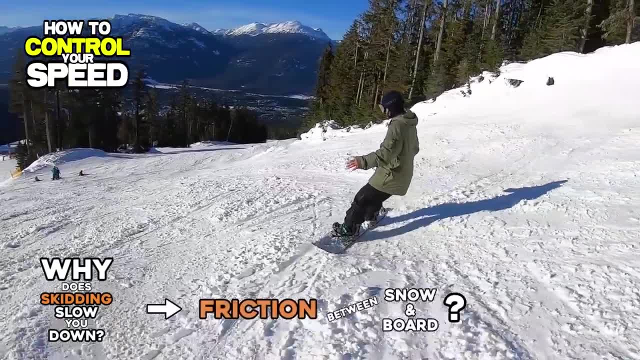 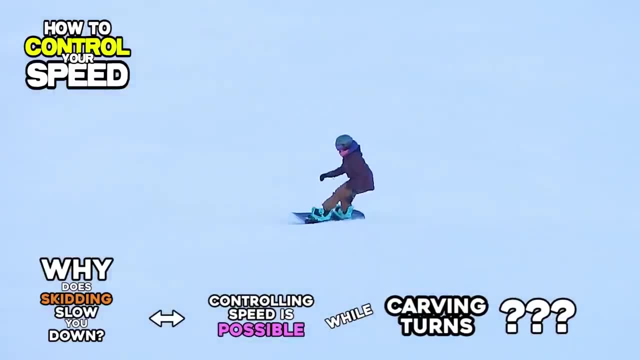 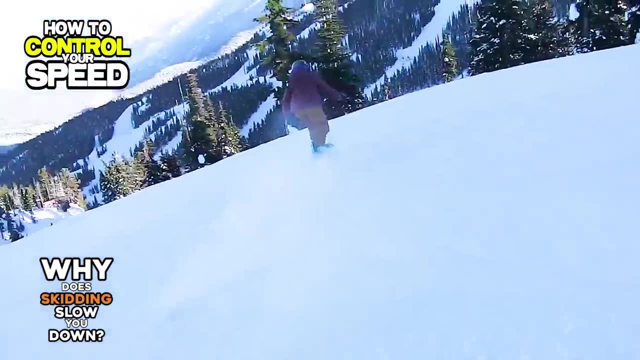 you down. When you skid, there is friction that is created between your board and snow. But here is the other truth: We can control speed even while carving. As you know, there is no skidding while in carving turns, but controlling speed is certainly possible When speed is. 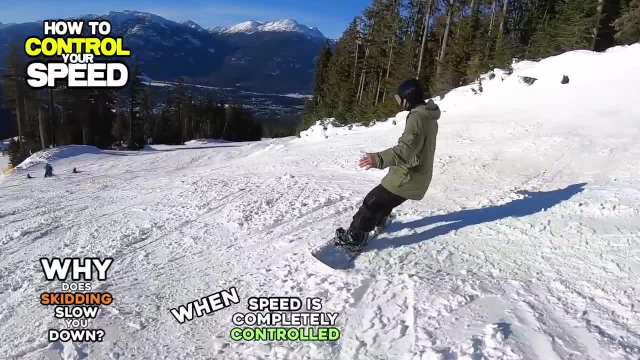 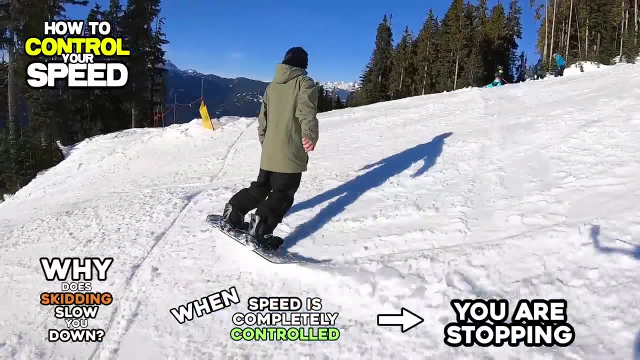 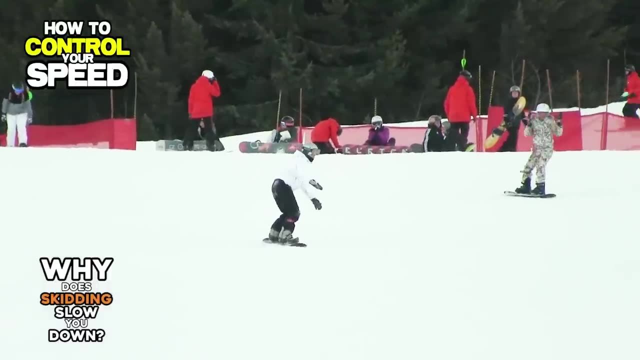 completely controlled and dominated while riding. what state is it? Yes, it's when we stopped and are standing still on the hill Because we will stop after slowing down. this state is the final result after controlling speed. Now let's try to bridge the gap between speed and speed. 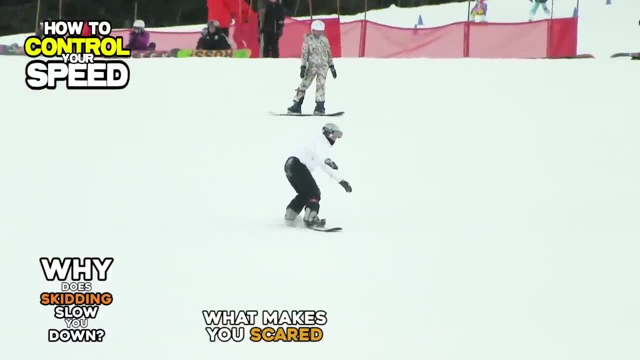 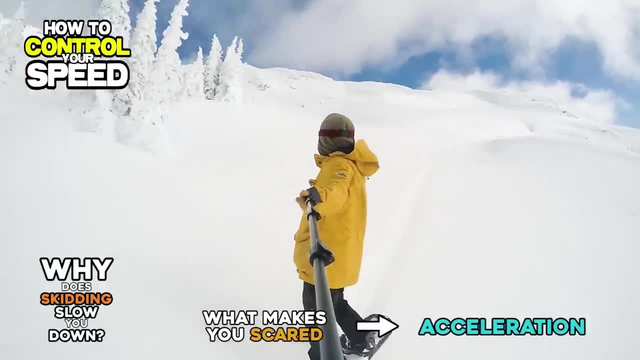 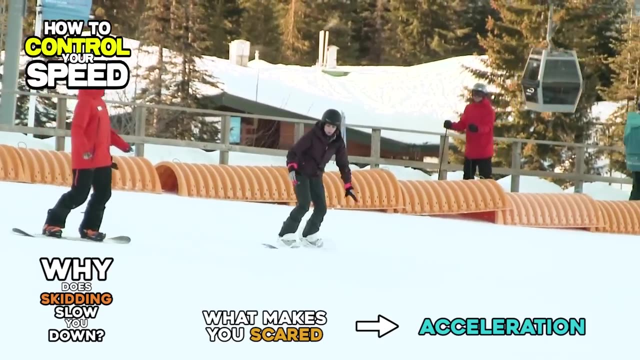 Why are you scared when you need to control speed? It's because you are feeling acceleration. If you can keep a steady speed, even while sliding straight down the hill, you won't be scared. But since your board is pulling down the hill while your board is pointing down, even a little, you'll. 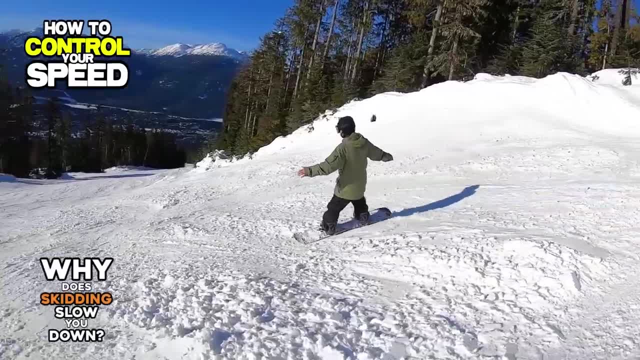 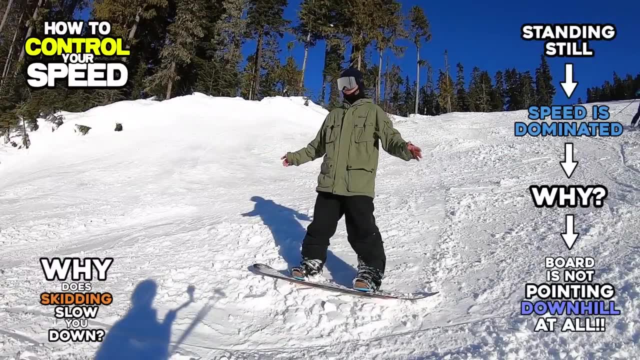 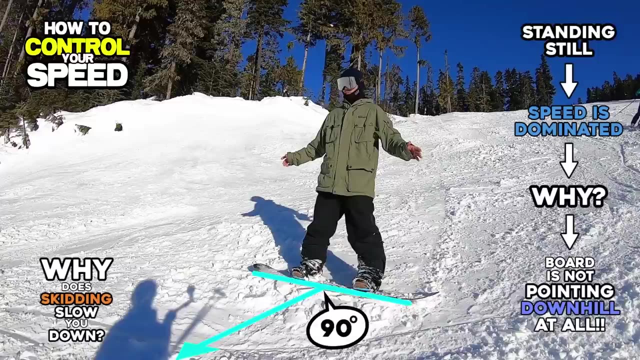 be adding more speed thanks to the gravity. Now let's think about why you can keep standing still on the hill while stopping. It's because your board is pulling down the hill while you're riding. In other words, your board is perpendicular to the hill. Yes, this is the answer for this. 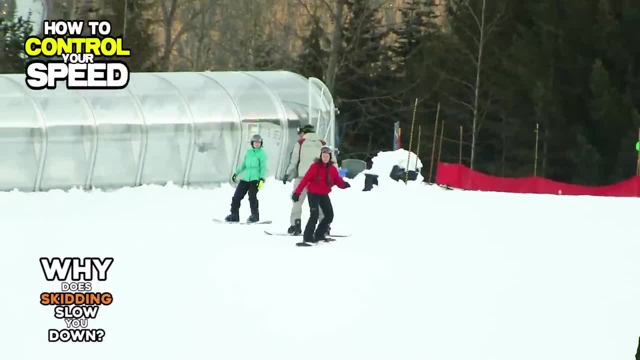 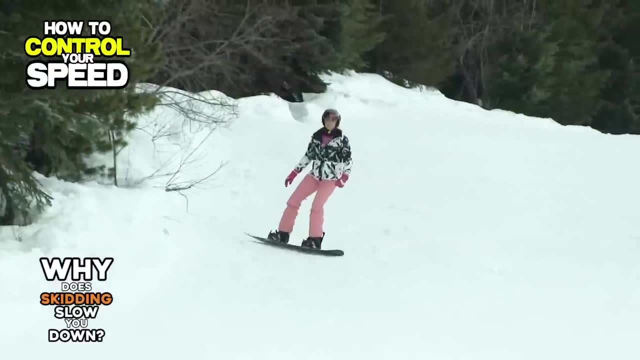 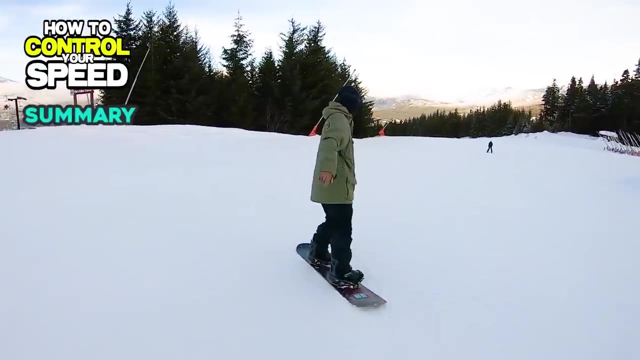 tutorial. When your board starts pointing down the hill, you will gain more speed every second. But if your board is not pointing down and perpendicular to the hill, you won't be accelerated. So you won't be scared. Here is the summary for this lesson. If you want to control 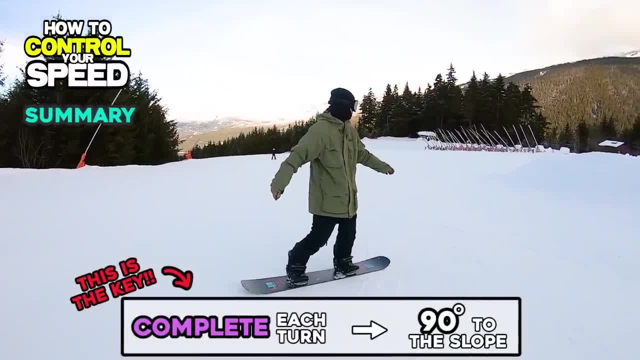 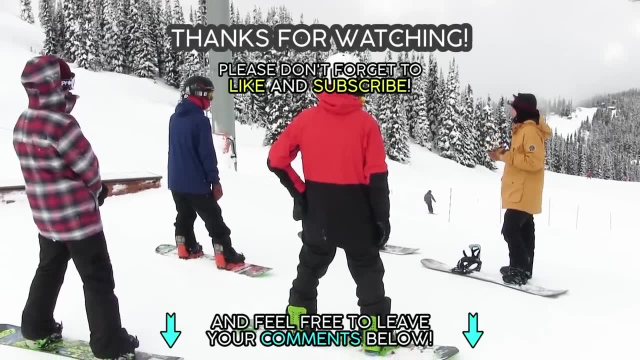 your speed while riding down the hill. you can control speed even while sliding straight down the hill. Complete each turn as your board gets more perpendicular to the hill. Please don't forget to like and subscribe to our channel, and feel free to leave your comments below.